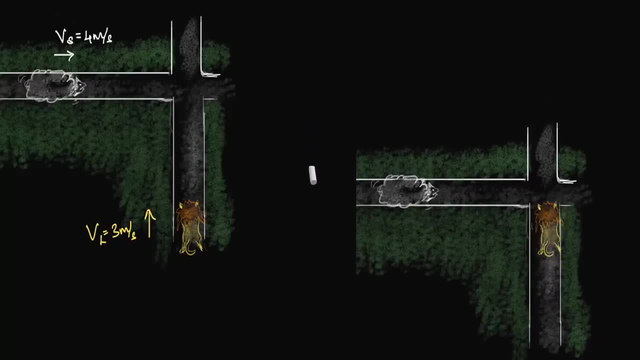 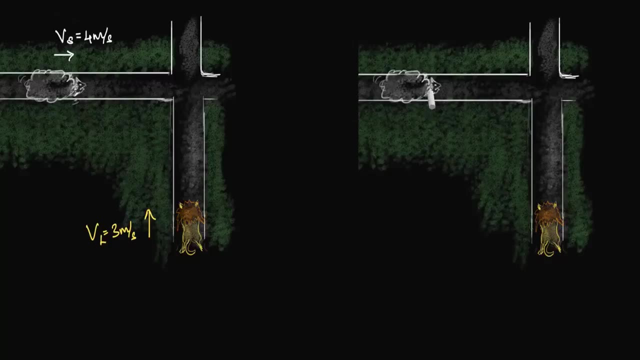 And if you have, if you have used GPS, then you see something very similar, right, You don't see yourself moving, You see the rest of the world moving. Now comes the big question: What will the lion see the sheep doing? I mean, think about it. 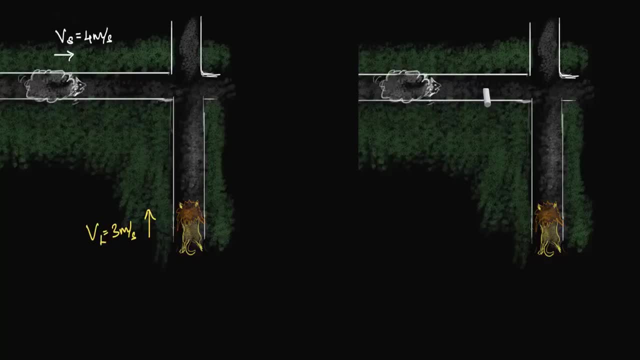 The sheep is moving four meters per second on the road, on the ground, But the ground itself is traveling backwards three meters per second. So to figure out the relative velocity of the sheep seen from the lion's point of view, we will wait for one second and figure out where sheep ends up. 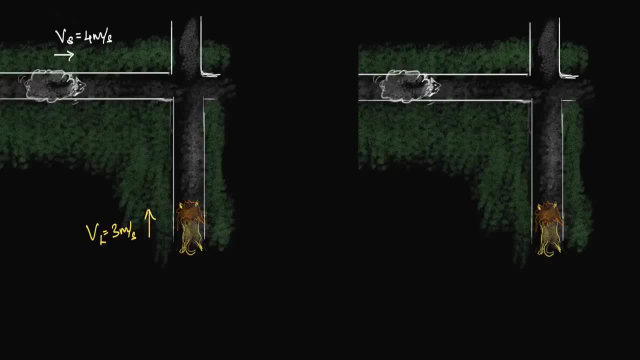 All right, Let's do that. So in one second we would see that the sheep would have traveled four meters on the ground. Right? So let's just write that down on the ground: The sheep would have traveled four meters. Here it is. 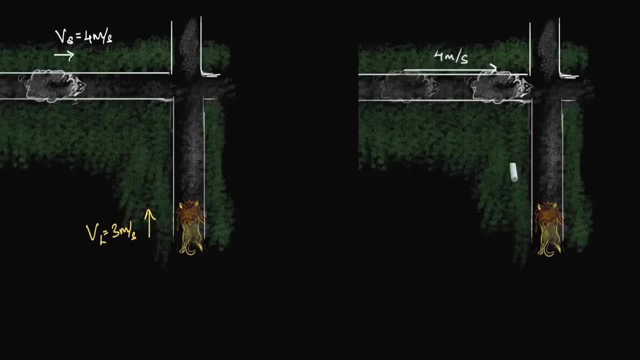 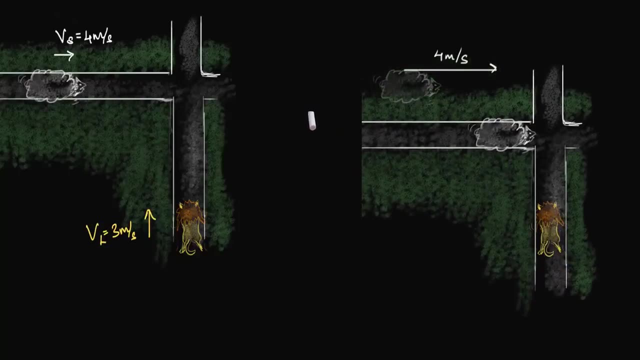 Four meters on the ground per second. But in that one second you will also see that the road and the sheep would have gone downwards, downwards, three meters. OK, so let's put that in as well. So the road and the whole ground. 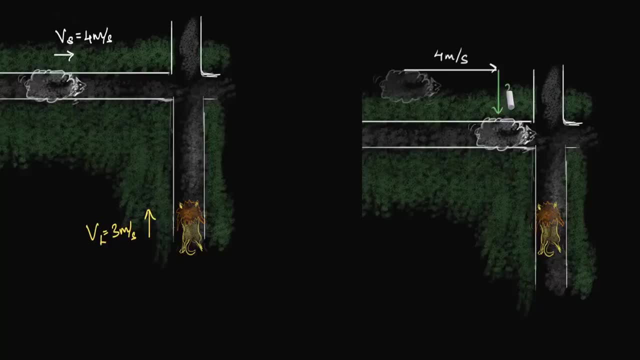 Whoops, All ground goes three meters in one second. So now here comes the big question: How much did the sheep move? Well, notice, the sheep was initially over here, but now it's over here. So if you look from the lion's point of view, the sheep has moved in this direction, this way. 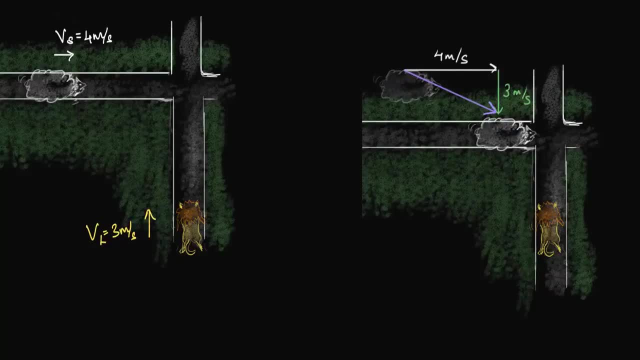 So this means that the sheep is no longer traveling towards the right. Instead, the lion would see the sheep moving this way, this direction, That is the direction of the velocity of the sheep, And I think that's a good question, And at first it might sound a little little weird as to you know, why would the sheep be doing that? 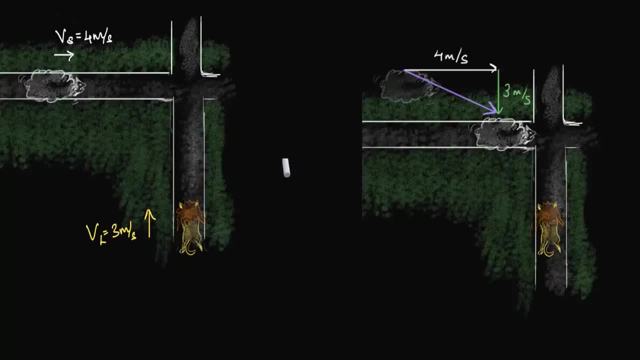 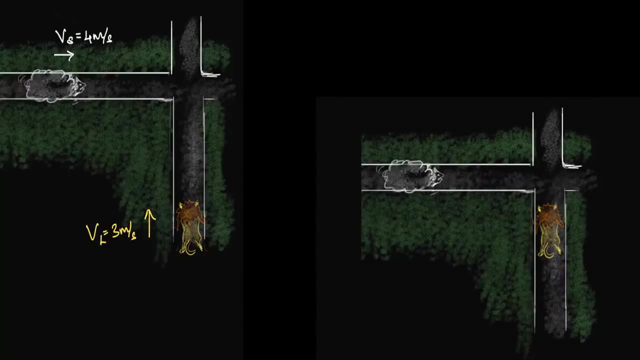 But let's play an animation to really convince you that that's really what's happening. So here it is. Here's the perspective of lion. All right, This is not very convincing, is it? OK, let's look at it one more time. 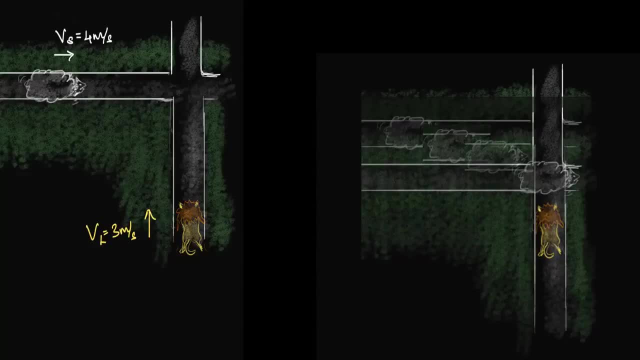 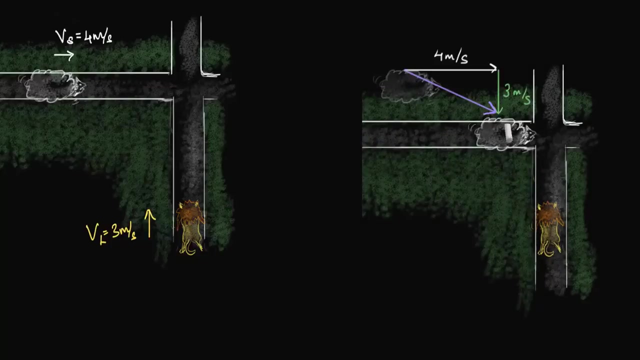 This time we will see some ghost images. Ah, you can clearly see now that the sheep is indeed moving at an angle, isn't it? So watch it over and over again until You really get convinced about this. All right, OK, now the next thing would be to calculate this. 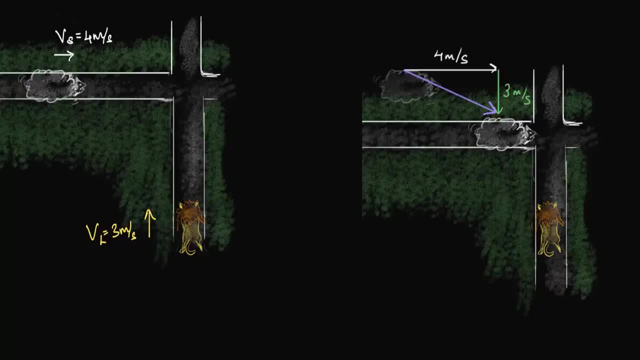 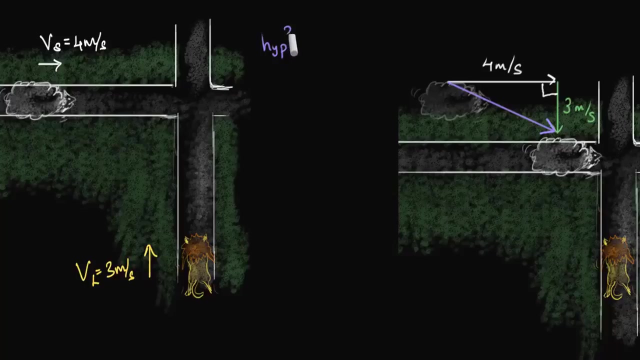 How much is this distance? Well, this is a right angle triangle And in right angle triangle we can use the Pythagoras theorem. This is our hypotenuse, So we could say the hypotenuse squared. The Pythagoras theorem says the hypotenuse squared is equal to the sum of the squares of the other two sides. 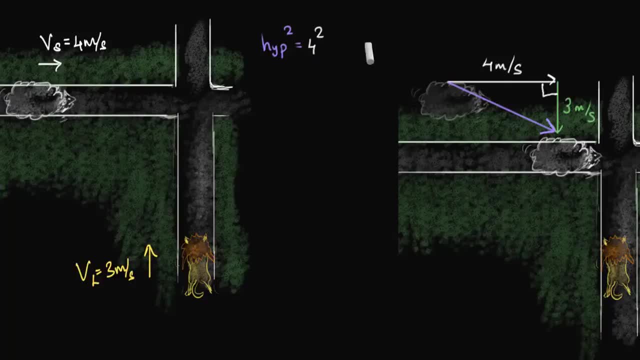 So that should be equal to the Square four squared plus three squared, And that gives us 16 plus nine, which is 25.. Or the hypotenuse turns out to be the square root of 25, which is just five, which means this length is five meters. 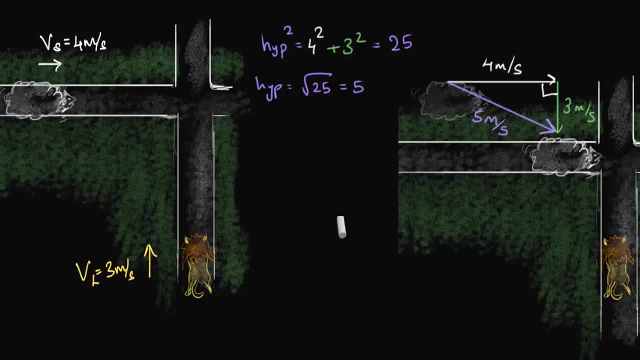 And this happened in one second Right, So we could say it's five meters per second. This means that the lion sees the sheep traveling five meters This way in one second. In other words, the relative velocity of the sheep as seen from the lion's perspective is five meters per second this way. 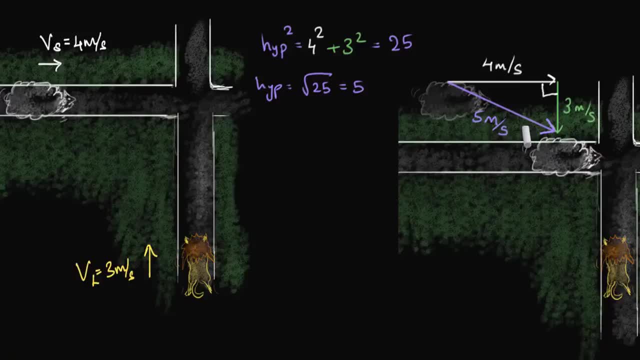 All right. Now, since we're talking about velocity, it's not just the magnitude, We also want to calculate the direction. I mean, no, we understand the direction is this way, But what exactly is this direction? So we can answer that by calculating the angle. 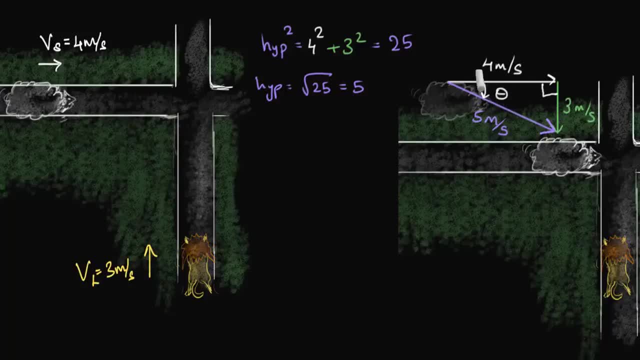 So let's calculate this angle, for example. How much is this angle? So We can use trigonometry, we can use sine cos. we usually prefer to use tan. It's not a necessity, You can use anything you want. 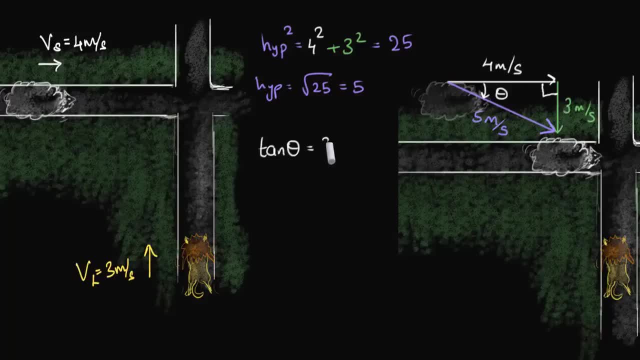 But if I use tan, we'll get the opposite side. three, Oops, let's, let's put the proper colors. Three divided by four, That makes theta equals tan, inverse of three. sorry, three divided by four, And there we have it. 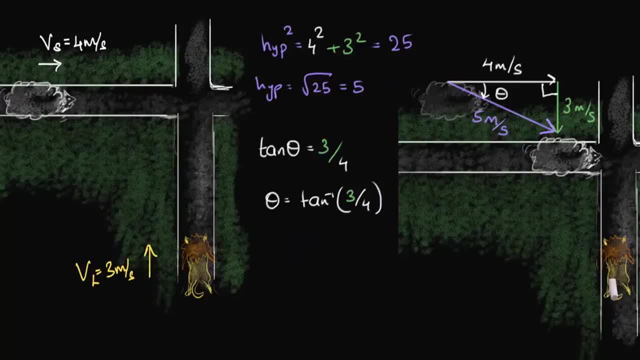 So if someone asks you now what's the relative velocity of the sheep as seen by the lion, we could just say it's five meters per second and an angle of tan inverse of three by four with the horizontal, or something like that. 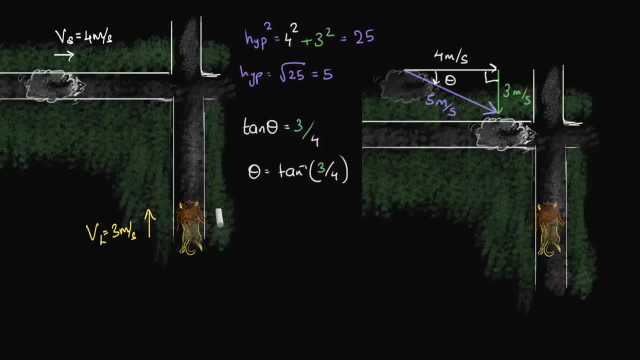 All right, Now let's put the whole thing, this whole result, in terms of symbols. Okay, Remember how we used to write symbols for relative velocity. Well, we are calculating velocity of the sheep with respect to lion, right? So we would write it as velocity of the sheep. 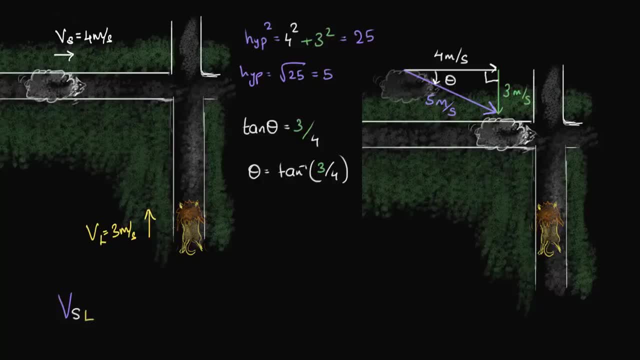 Sheep With respect to the lion, The only thing we have to do now is make sure that we put vector signs, because we are dealing in- we're looking at things in two dimensions, right? So we have to use vectors. And if you're not familiar with vectors or if you're uncomfortable with vectors, 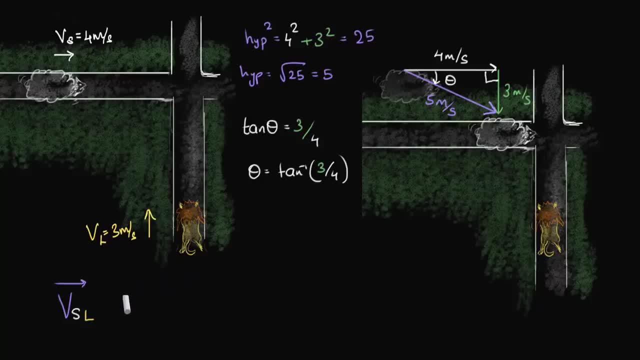 then it would be better if you could first watch those videos on vectors and then come back over here. So anyways, let's try to write this now. What is this equal to? This vector? is this vector which we have drawn five meter per second? 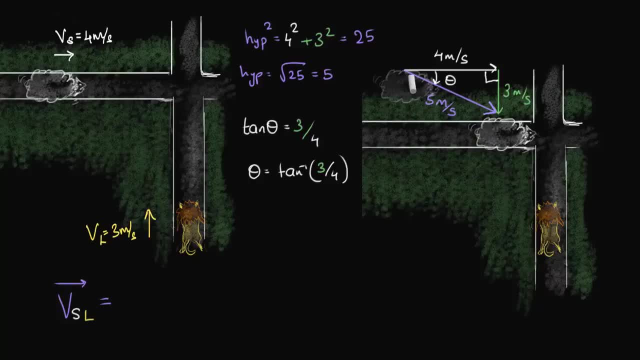 So how did we get? this is the question. Well, we added this vector and this vector. right, This is a triangle law vector addition. So we have to add the white vector, but white vector is just the velocity of the sheep as seen from the ground. 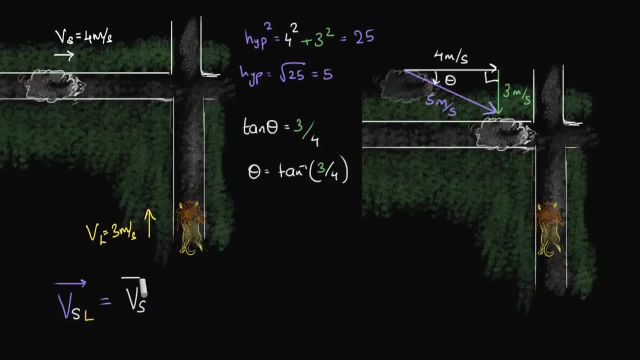 So that is equal to velocity of the sheep as seen from the ground, Plus because we are adding this vector. What is this green one? Ooh, that's the negative of this vector, right, I mean, since the line is going. 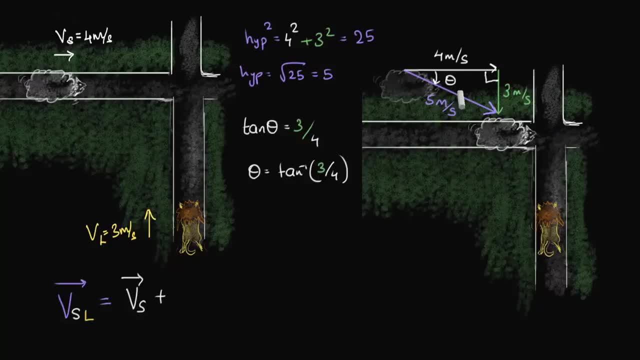 Upwards three meters per second. That's the reason the ground goes backwards: three meters per second from the lion's point of view right. So this would be the negative of the velocity of the lion as seen from the ground. And there we have it. 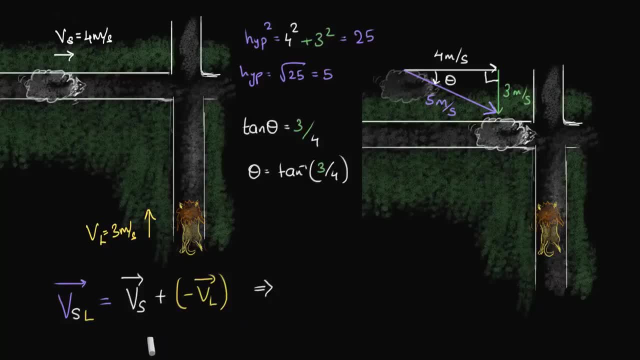 This is a general result. Just to make it more concise, we have a plus of a minus. We will rewrite this. rewrite this as velocity of the sheep with respect to the lion as velocity of the sheep Minus velocity of the lion, right. 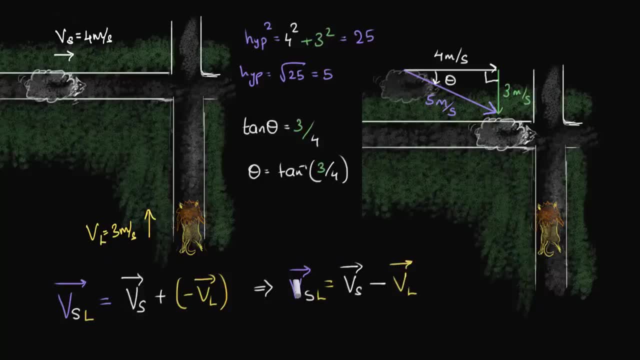 And this is the same as this. okay, And the reason I want to box this expression is because this is very similar to what we got in one dimension. Do you remember? in one dimension, we got VAB equal to VA minus VB. Well, guess what?